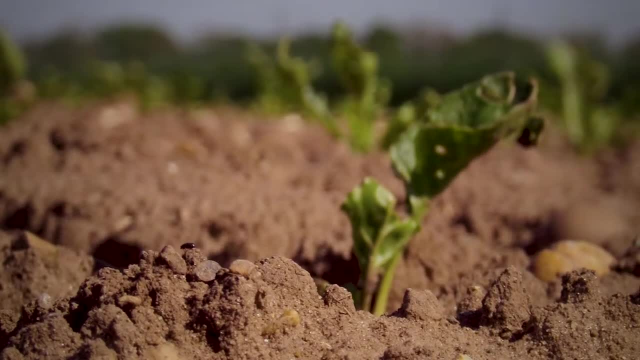 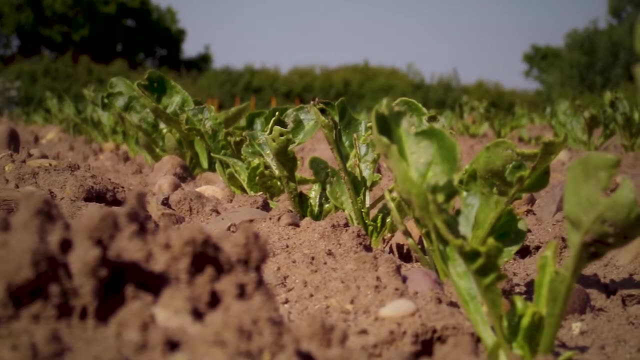 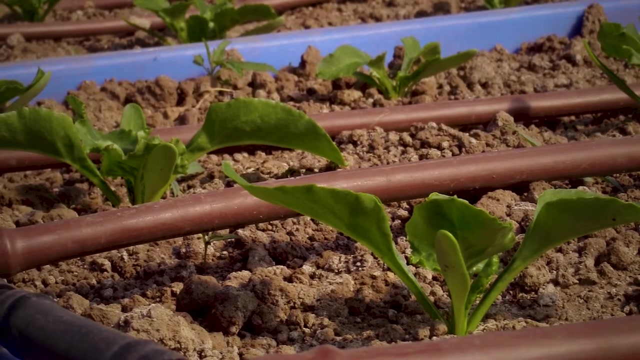 growers on the best way to manage their crop, and others are people working directly in the industry, such as for companies like British Sugar. So, while they might understand crop growth and development and how to produce the best yield today as conditions change in the future, for instance at the moment, 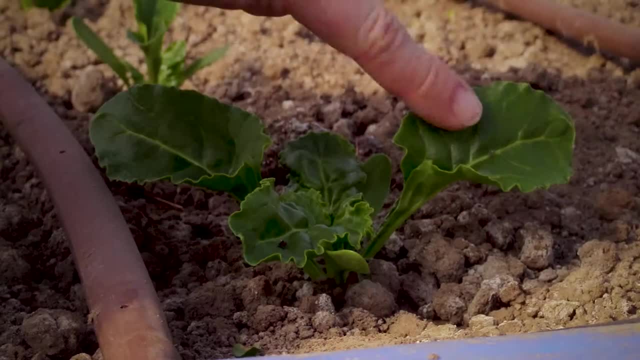 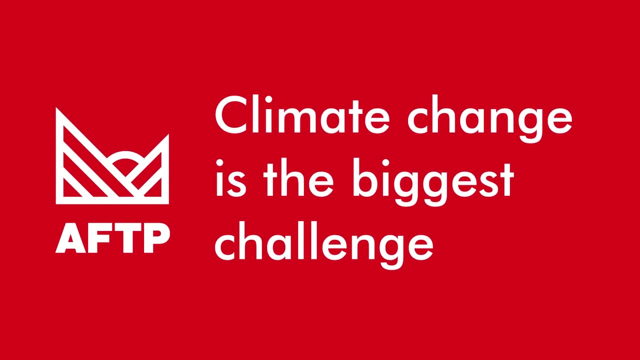 we haven't got the use of some of the chemicals we used to have. if you have a good understanding of the fundamentals of the crop, you can see how to change things when conditions change. Climate change is evidently the biggest challenge. we've got coming down the line and all of our crops are going. 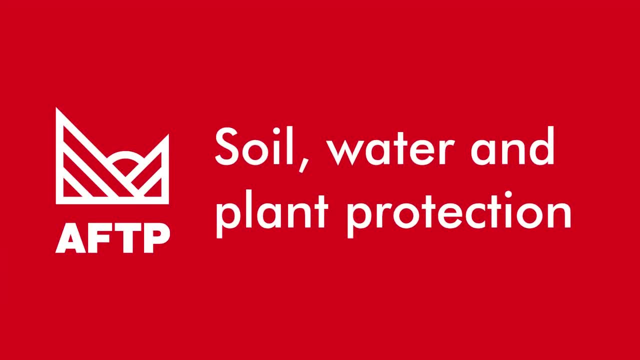 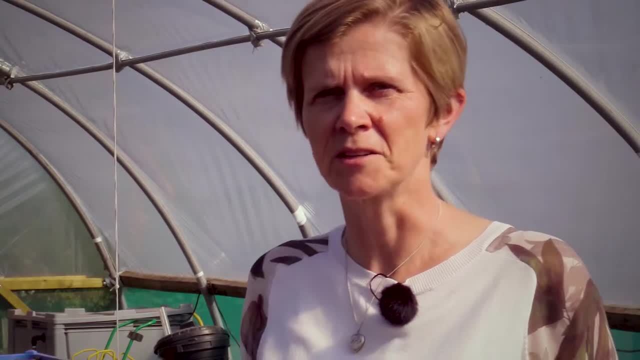 to have to to adapt to that, and sugar beet will be one of the UK crop producers. It's one of the crops that is most challenged because of the fact that it's grown on sandy soils which don't retain moisture very well, and it's sown in March just as the the rainfall. 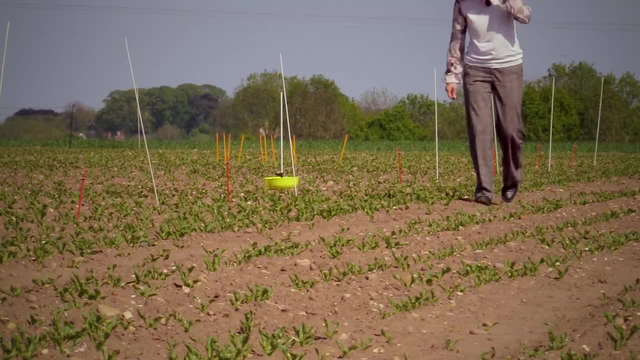 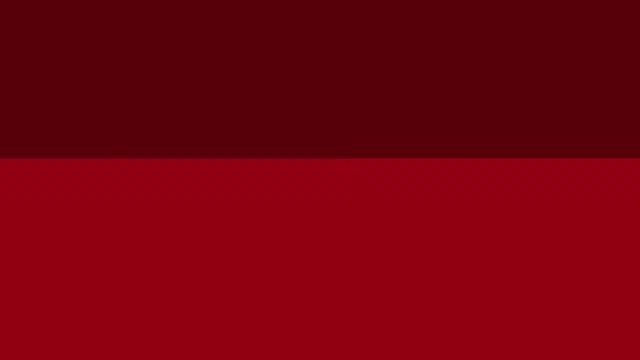 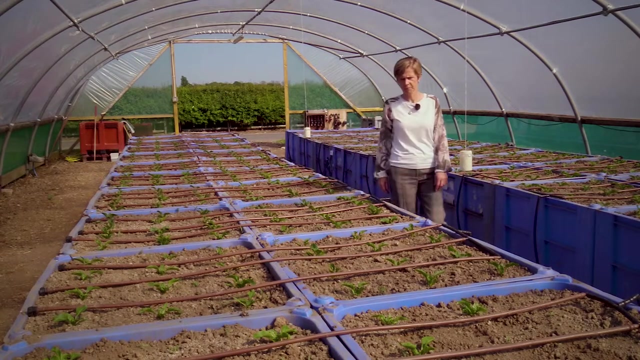 is likely to sort of peter out over the over the summer period, Times are very challenging and there's there are more risks coming down the line and as the chemicals disappear, we've got to be more prepared and more and plan further in advance for protecting the crops and relying on a mixture of biological 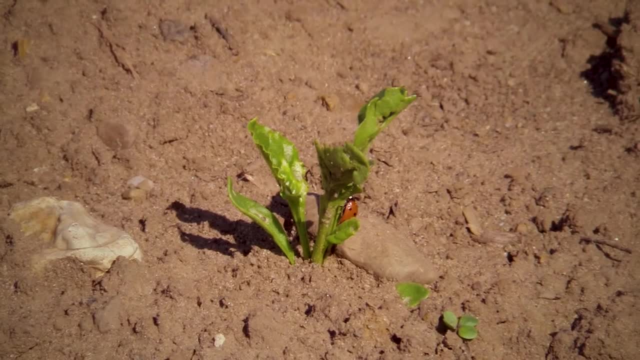 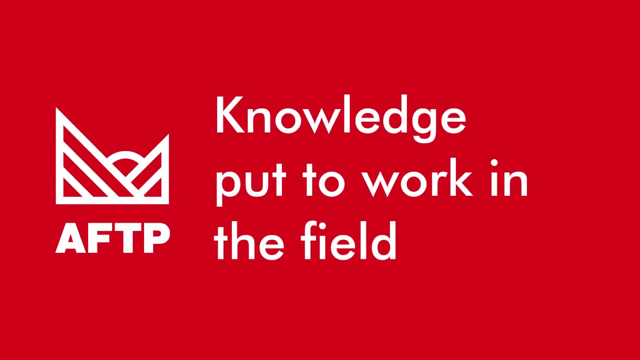 control. so the beneficial in all of these crops? I think we need to get more of the existing insects, like the ladybirds that we saw, to do some of the work for us. rather than previously, we him more of an armoury of sprays that we could, you know, could use. 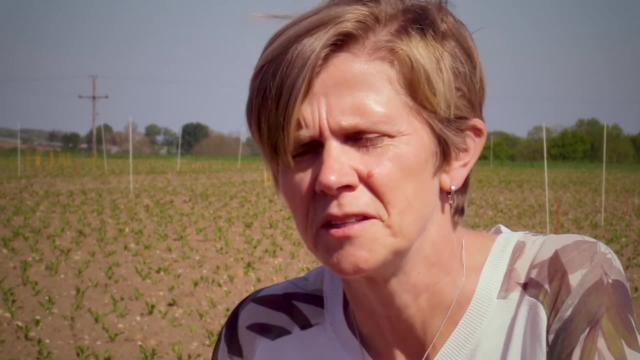 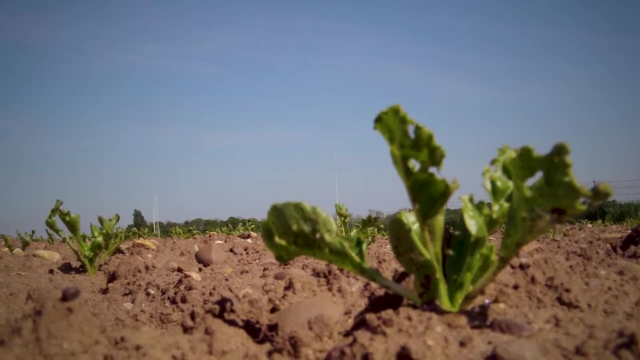 They shouldn't just go away with new knowledge should be new knowledge that they can apply in their role. and because it's done in a very discursive way, people can ask questions all the way along. and so, okay, we- how would I change it in my situation? and we often have conversations. oh, it's all very well if you're working on this type of farm, but on the farms I work on, the soil is very sandy, the nitrogen leach is through. how can I make it better? 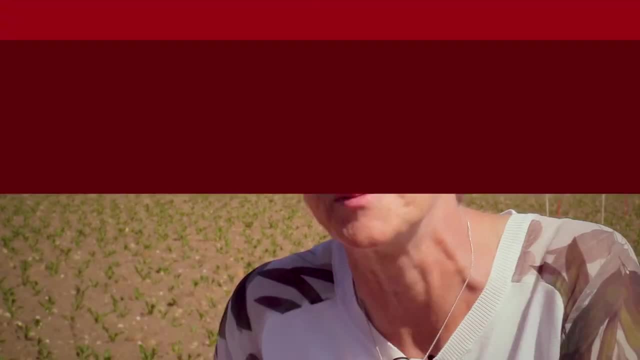 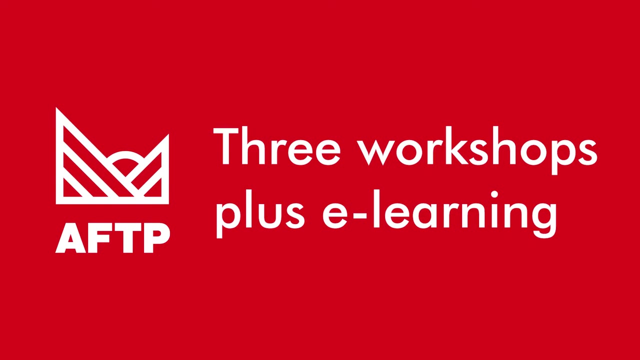 Now it's time to talk about. agriculture is very sandy, the nitrogen leaches through. how does it work for me? and we have those, those discussions and conversations. it's very much a blended course, so there's there's some e-learning and then there are lots of seminars with different contributors coming in. 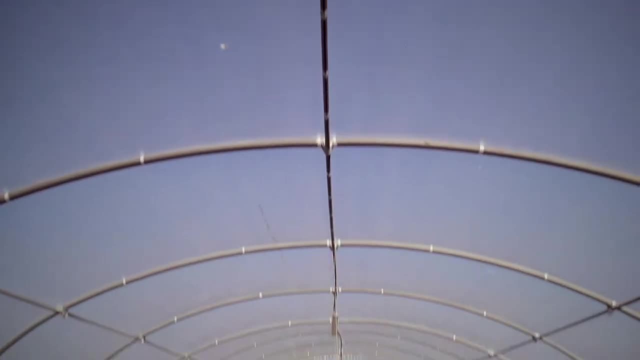 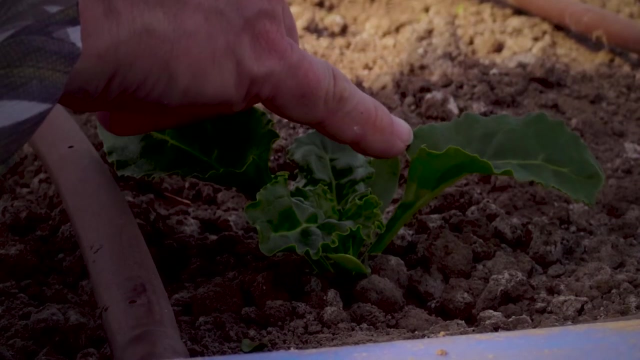 from the university, from industry, talking about their specialisms, and then we have practical classes. so coming out to the field or going into the laboratories where you can actually go and work out how to identify one aphid from another or see how the tests to identify viruses.